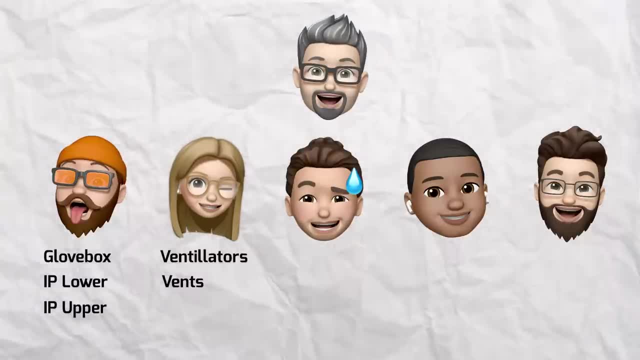 He decides to give Ashley the ventilators and vents, since she has the most thermals experience. He decided to give you the cluster bezel, speaker assembly and cup holders. Fourth, he gives Sam the steering column, display screen and gap hiders. Finally, he gives Theo the 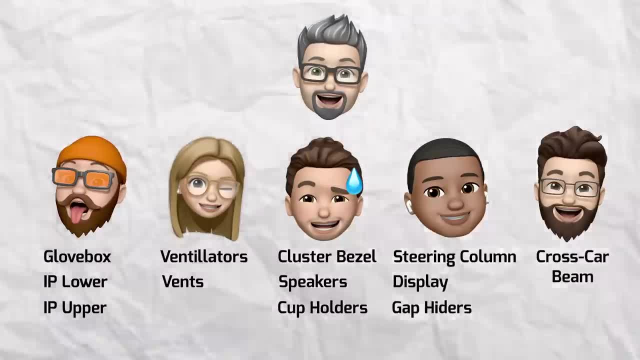 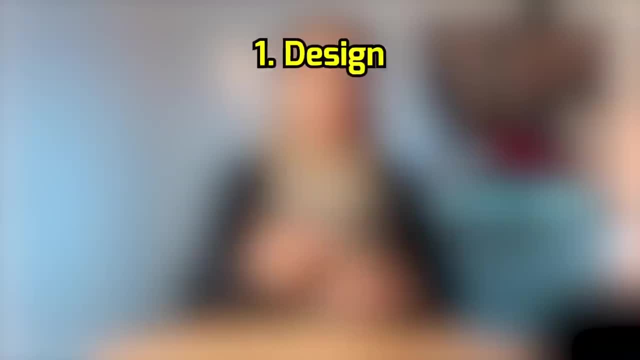 cross-car beam, which is the backbone of the instrument panel. Every mechanical engineer is responsible for the product lifecycle for the parts that they were assigned. The lifecycle includes six steps: design, development, review, testing, deployment and maintenance. Now within the product lifecycle, under the development stage. 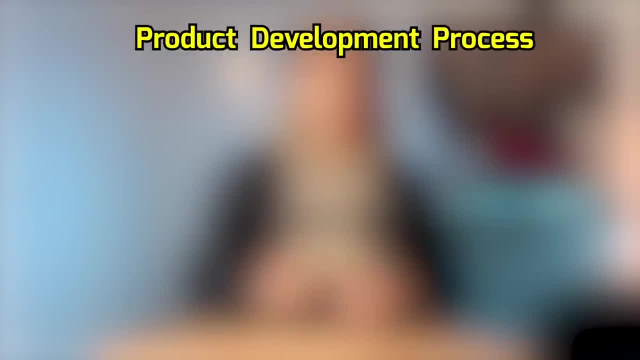 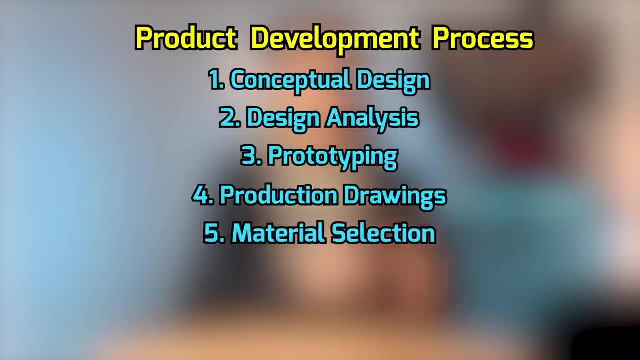 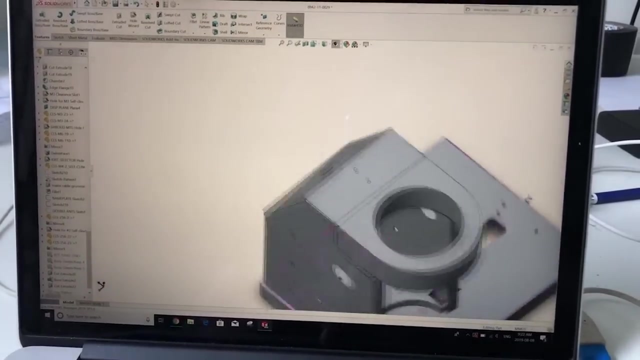 there is a product development process that we need to be comfortable using, and it contains eight steps: Conceptual design, design analysis, prototyping, production drawings, material selection, pilot production, production and QA. We use CAD software like SOLIDWORKS to do the design analysis. 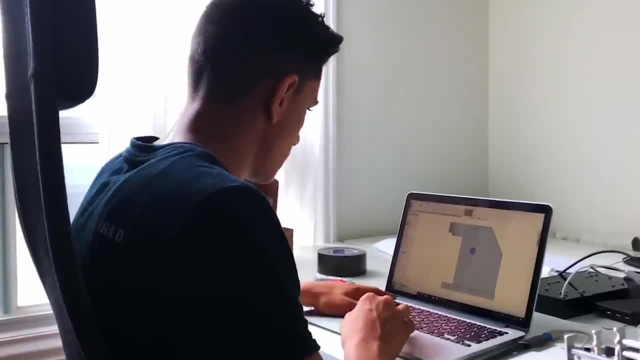 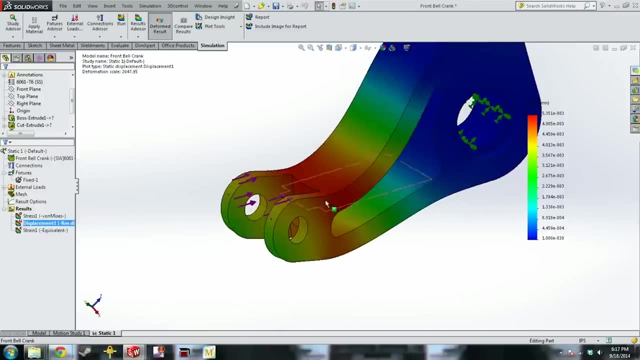 prototyping and production drawings. For instance, we'll use SOLIDWORKS simulation to do some finite element analysis on some parts to see how they'll perform under heavy loads or under changing temperatures. We can then continue testing our design by creating 3D printed. 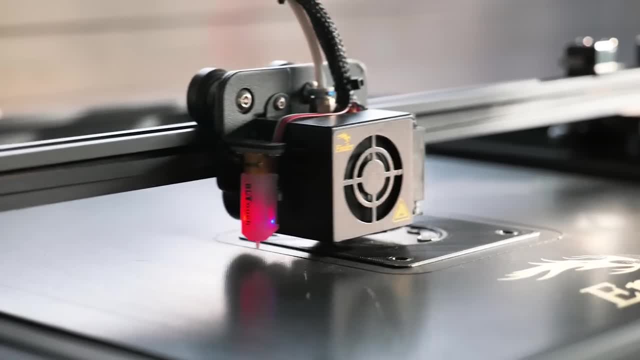 prototypes and once we're content with our design, we'll go into creating production drawings. These drawings look like this and would get sent out to external suppliers, who will give us feedback and we'll be able to use them to create our own production drawings. We'll also be able to 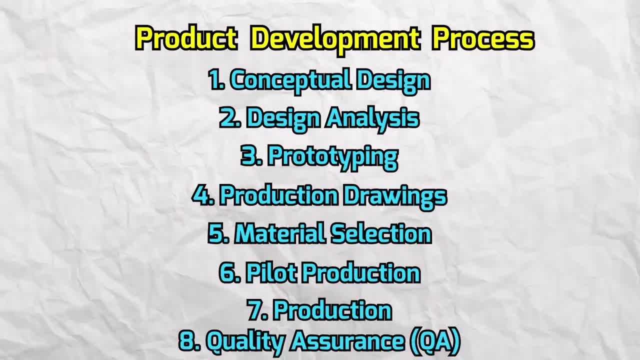 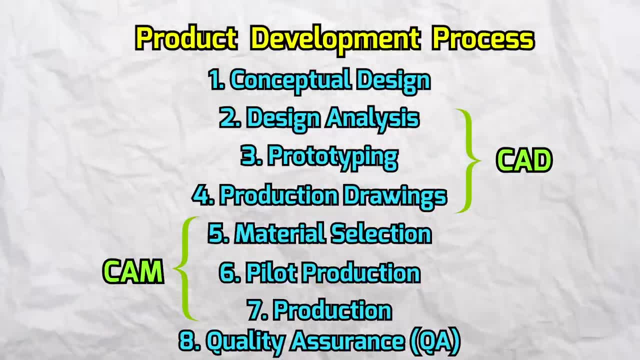 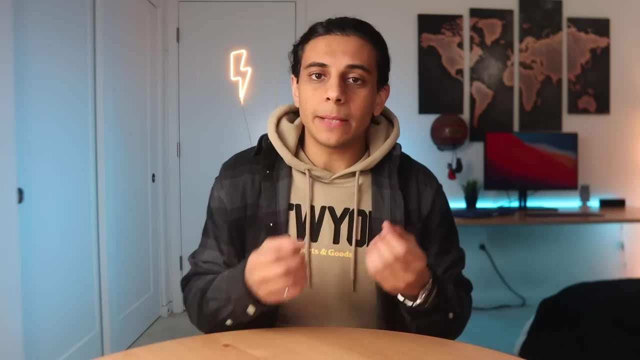 get feedback on how easy it is to actually build it. The next three steps fall under the computer-aided manufacturing category, or CAM for short, where we convert CAD models into information that can be used by machines on the shop floor in order to transform raw materials into finished products. Now, sometimes, instead of calling this position a 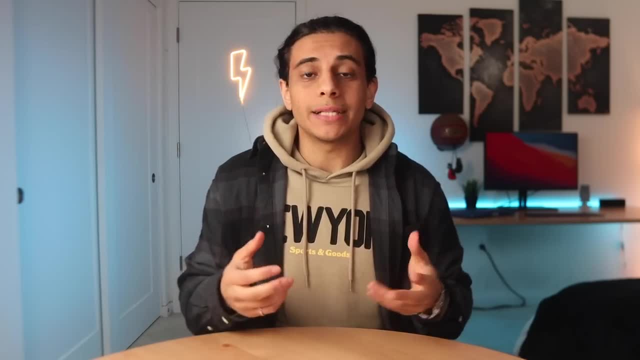 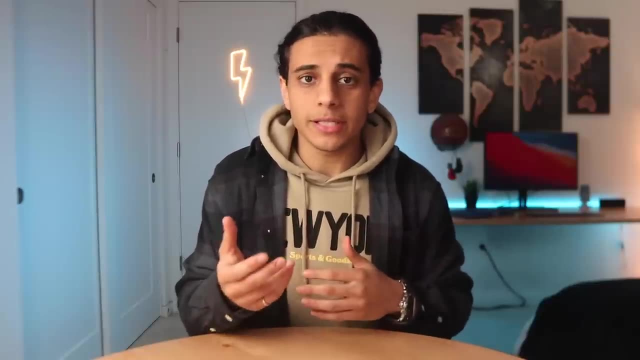 mechanical design engineering role. we can refer to it as a product design engineer. Usually, companies that are more consumer electronics-focused will kind of use that title, like Apple, for example, but regardless, they both do the same thing. However, keep in mind that there is a difference. 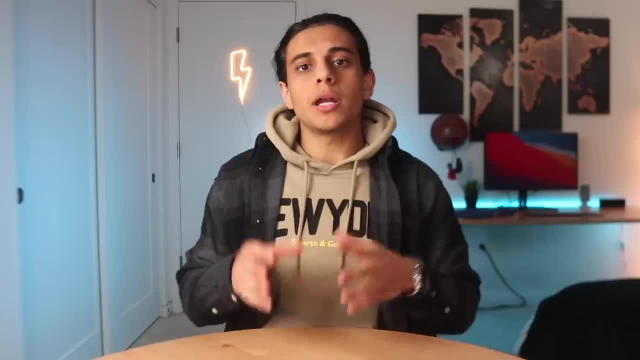 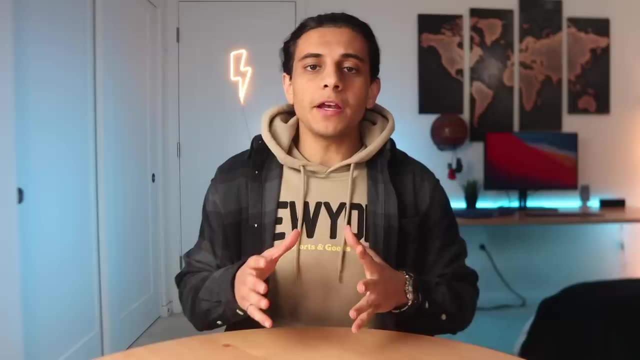 between product designers and product design engineers. A product designer is someone who designs a physical product based on user needs, and they're really just starting off with pencil sketches. They figure out what the general look and style of the product will be and all their 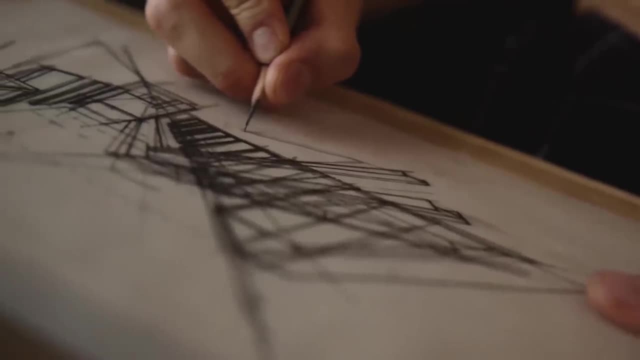 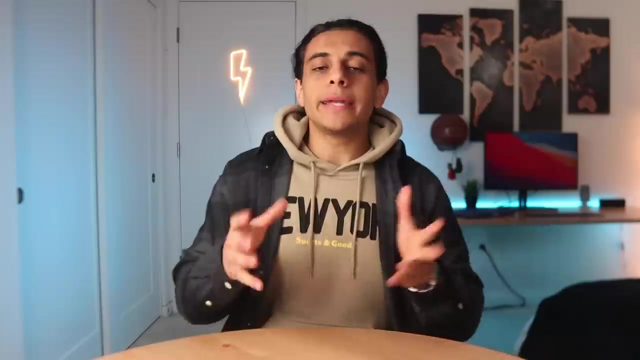 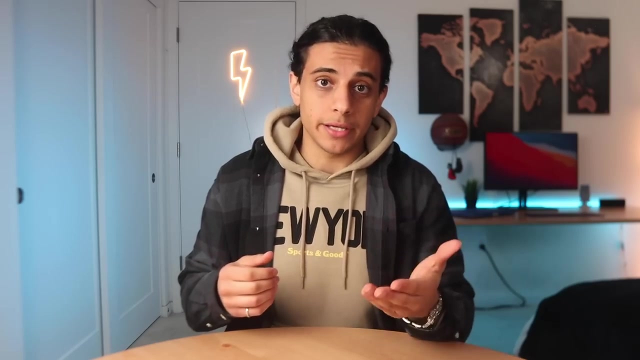 sketches explore all the materials, colors, shapes and features that are possible. The output of their work is usually sketches, renderings, models or non-functional prototypes. Now, a design engineer's someone who designs the engineering or manufacturing aspect of a design that was given to them by a product designer. They're usually using 3D CAD. 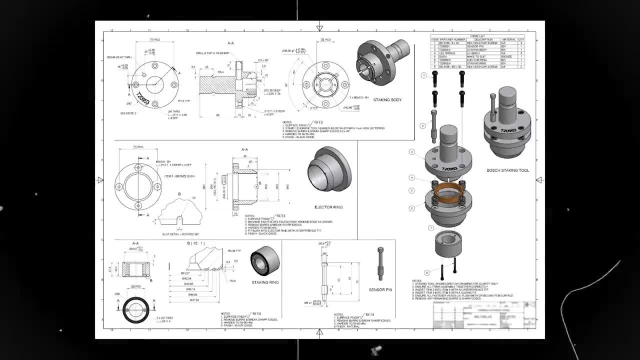 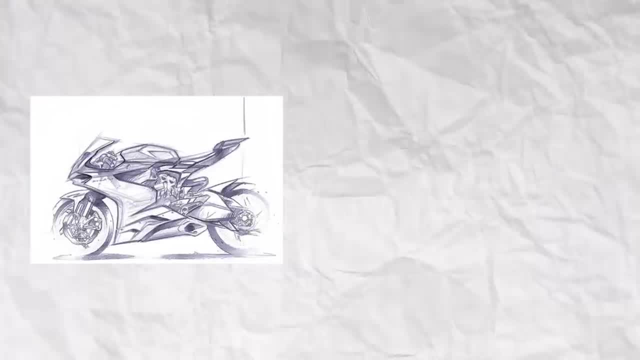 software to do so. The output of their work is usually technical drawings, fixtures or tolerances. For example, when a product designer designs a bike, it will look like this. On the other hand, when a product design engineer does it, it'll look something like that: 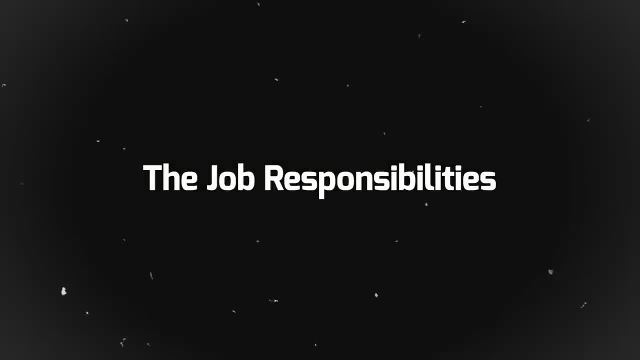 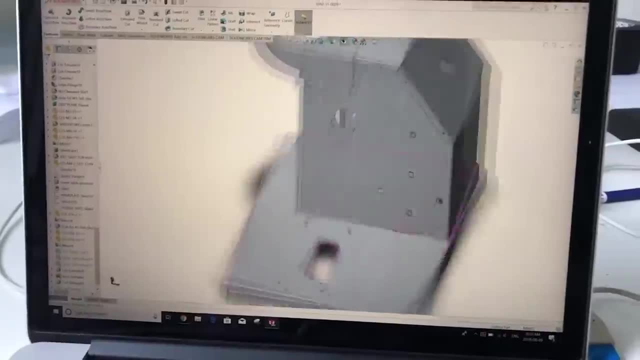 Now let's look at some of the responsibilities that you have as a mechanical design engineer. First, you will design parts, components and assemblies that meet the requirements of your design projects. Second, you will create CAD models, engineering drawings, building materials. 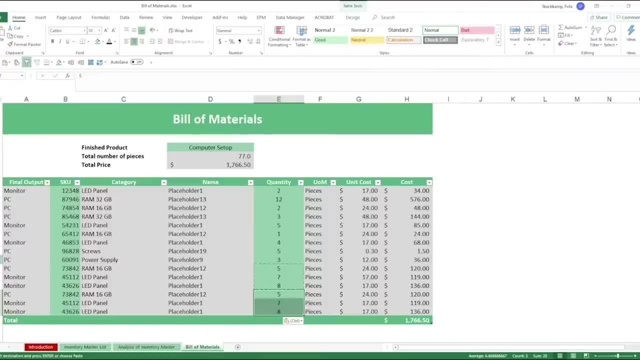 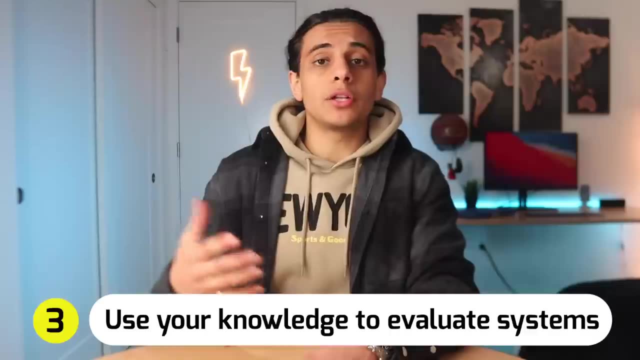 or BOMs for short, and testing and assembly documentation. This helps make the product feel real and allows you to design something that can actually be built. Third, you can find yourself using your knowledge of material science or thermodynamics to evaluate mechanical systems. 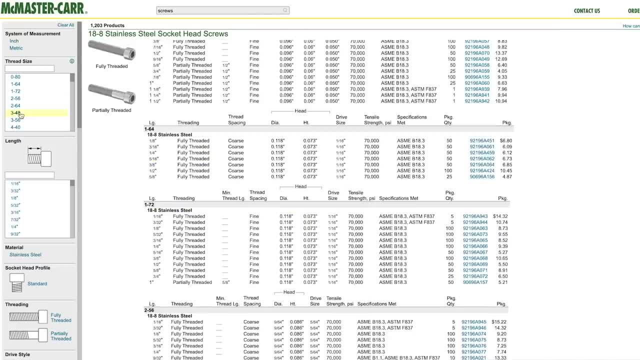 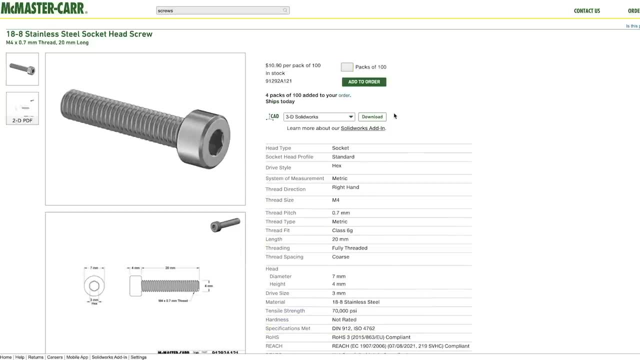 Fourth, you can be helping out with the product sourcing and purchasing of the parts that will go into your design. That means, if you need sheet metal to be bent a certain way or specific screws, you need to go and buy it yourself. Fifth, when things go wrong, you'll probably need to undergo root cause. 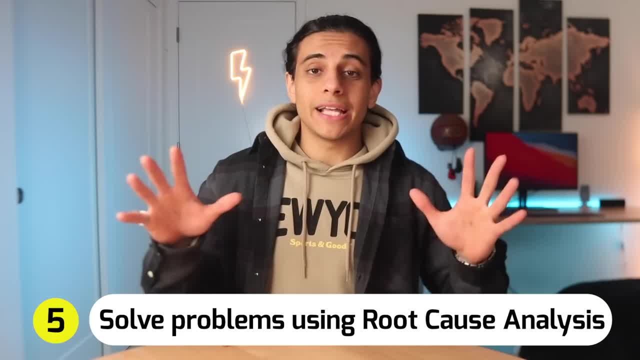 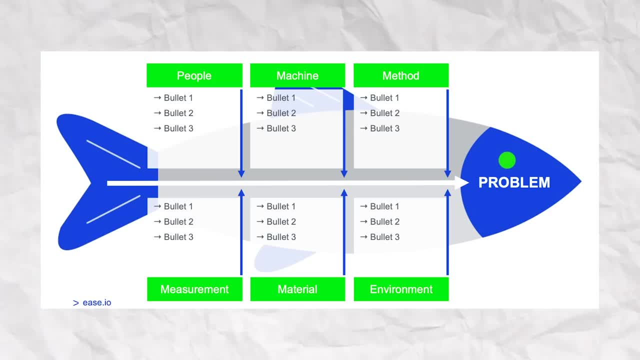 analysis to figure out the root cause of a problem. There's a whole science behind this and there's a bunch of different root cause analysis methods that you can use to do so, like FMEA charts, fishbone diagrams or the five whys. Sixth, you may find yourself participating in 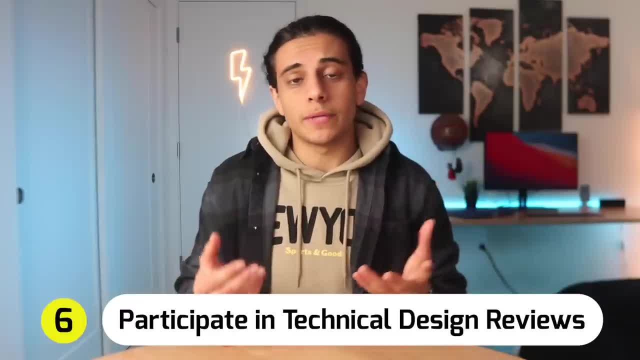 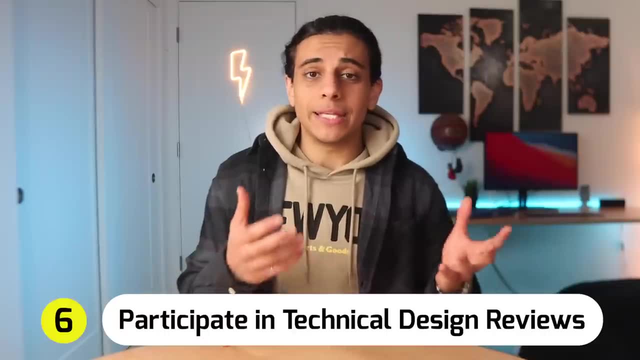 technical reviews. This means that if another mechanical engineer finished one of their designs, they'll share it with you for some feedback. You may propose a better material that they could use, or maybe you feel like their design isn't really easy to assemble, so they propose a better solution. These are just the six main responsibilities. 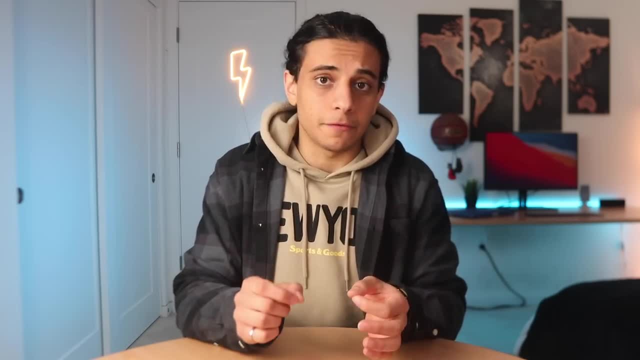 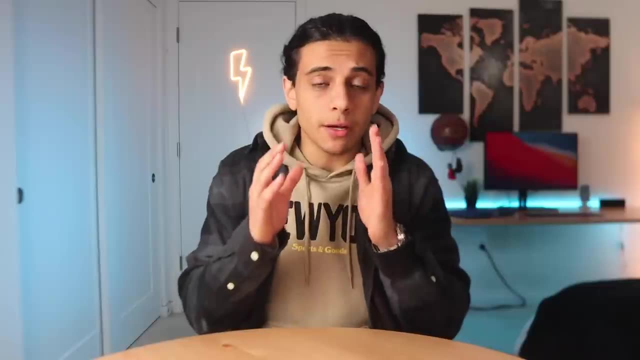 but obviously every single mechanical design engineering role is a little bit different. Smaller startups or companies may have you be a lot more involved, with a lot more responsibilities, but larger companies will have you just hone in and focus on one specific aspect of mechanical engineering. Now, if you're working on a part or product that is relatively new and is in the 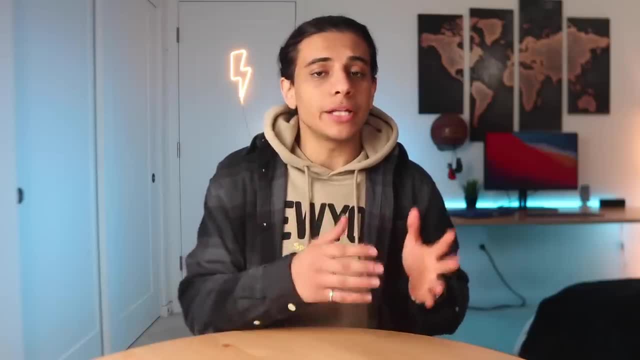 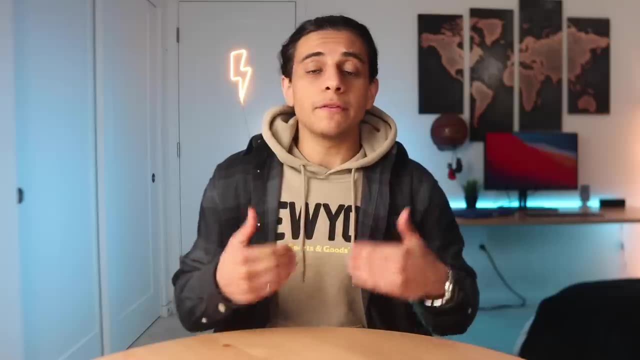 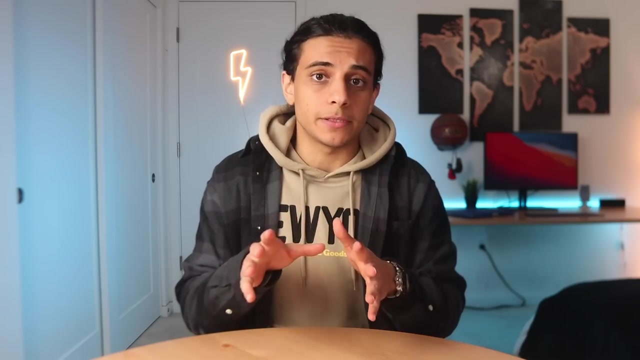 earlier stages of the development process, you may have to undergo the engineering design process. It starts off with product designers, who'll send you sketches or digital surface models of what they want the final product to look like and feel like. Their models are usually non-functional, and it's our job to bring these models to life in a few steps. 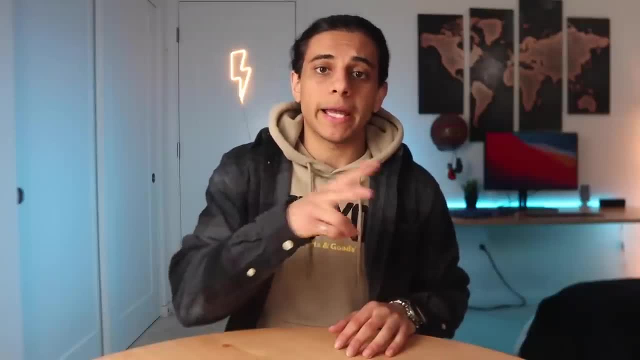 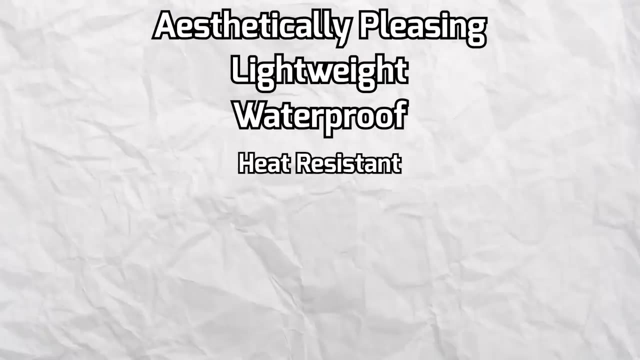 First, we need to break down the part we're working on into its components. Second, we need to figure out what requirement each component has. That can include things like aesthetically pleasing, lightweight, waterproof, heat-resistant, strong, low-cost, securely mounted, aerodynamic, etc. 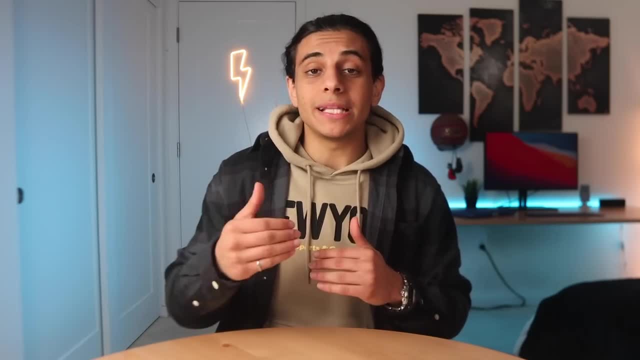 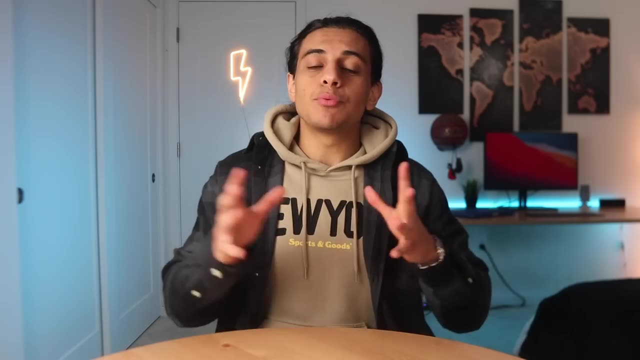 Every requirement must be met, but sometimes achieving one requirement means sacrificing on another, So things can get a little messy. For example, let's say you're designing this component for one of the new cars that you're working on. The product designers gave you information on what the part will look like. 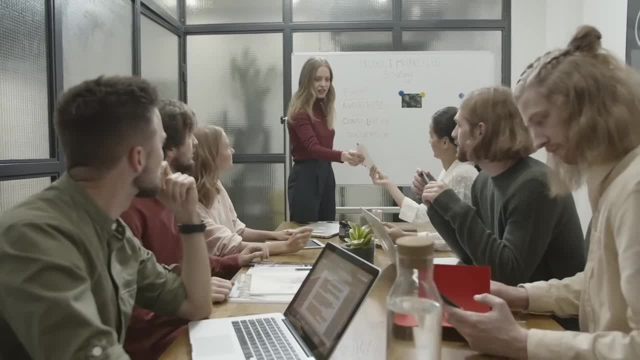 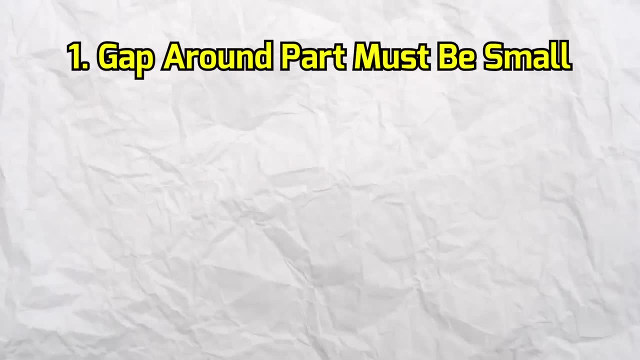 on the outside. then all the mechanical engineers sat together to create a bunch of product requirements. For instance, some of the requirements were that the gap around the part must be small enough so that it doesn't look ugly. it also can't be taken off too easily. 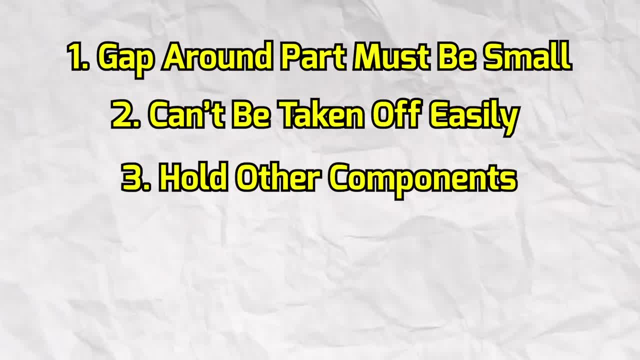 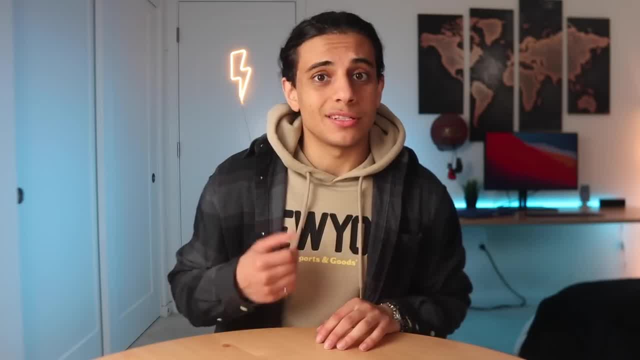 it needed to hold other components and easily attach to its surroundings. it also needs to look good and there was also some mass and cost requirements. With that, you'll need to start asking yourself questions like: how do I mount this part? Do I use tape, Magnets, Screws, Clips? If I use clips, 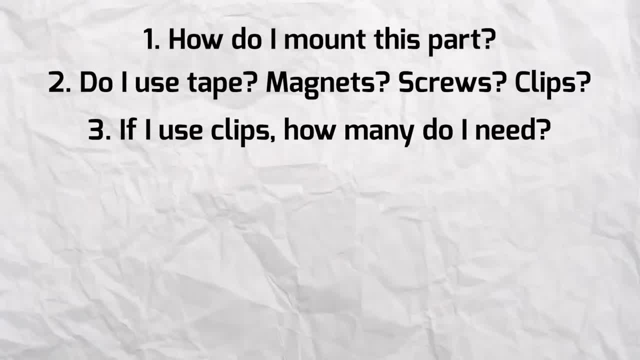 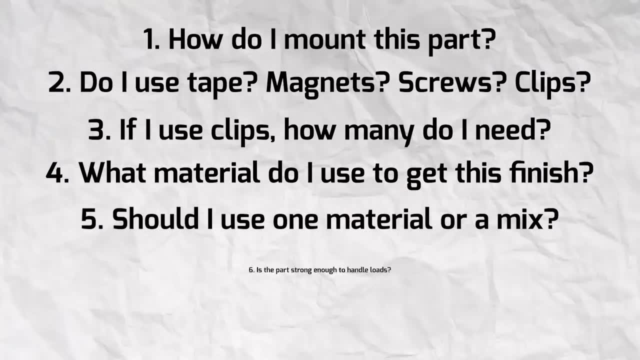 how many do I need and where should I place them so the part can be securely mounted? You may also ask yourself: what material should I use to get this nice finish? Should I use only that one material, or should I use a mix of materials? 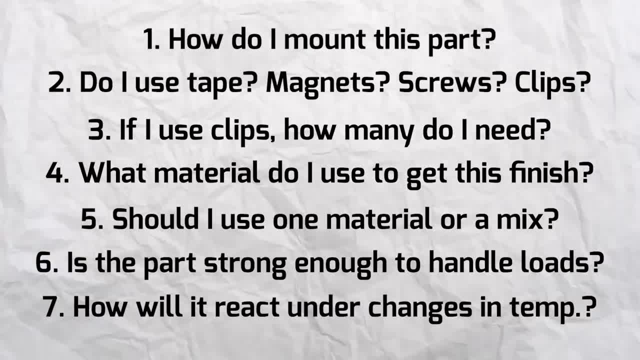 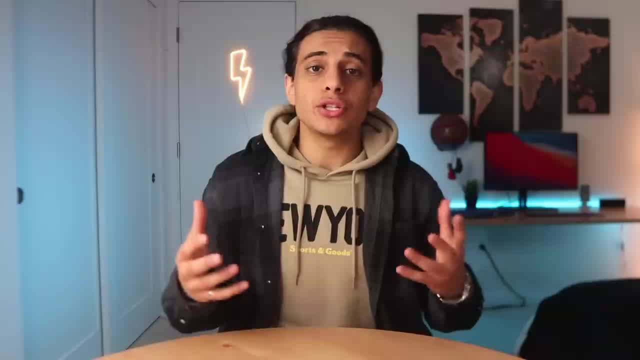 Will the part be strong enough to handle additional loads? How will they react under changes in temperature, For example, when it's been out in direct sunlight for too long? As you answer these questions and you make decisions on the parts, you'll need to start asking yourself. 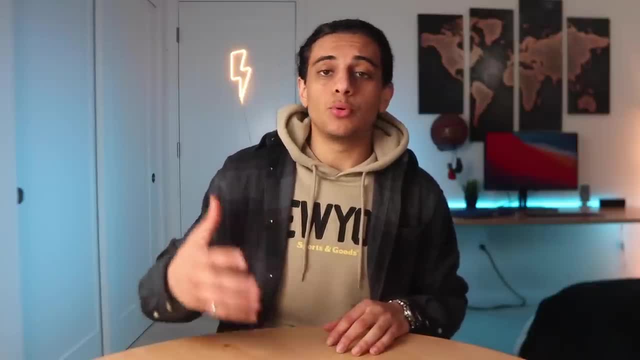 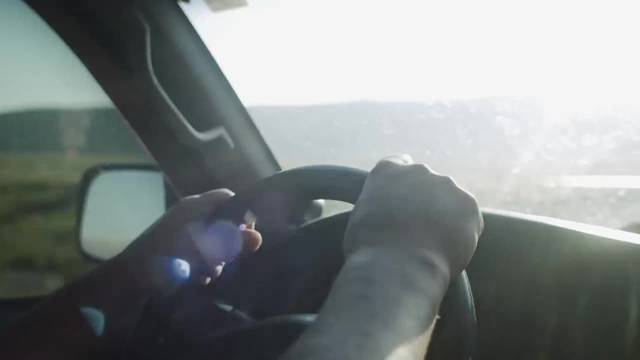 how do I mount this part? Do I use tape, Magnets, Screws, Screws, Screws. You'll need to implement some root cause analysis to basically predict how things will go wrong, For example, if you plan to mount this part using an adhesive. but you know this part. 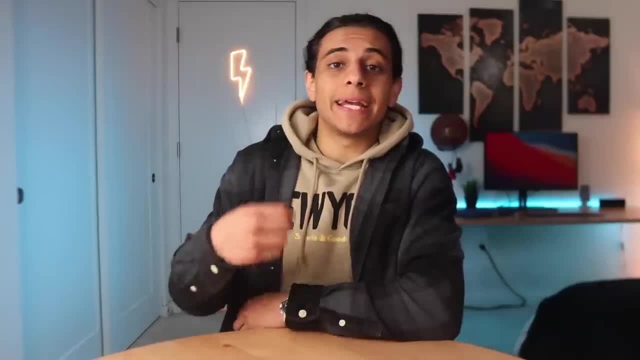 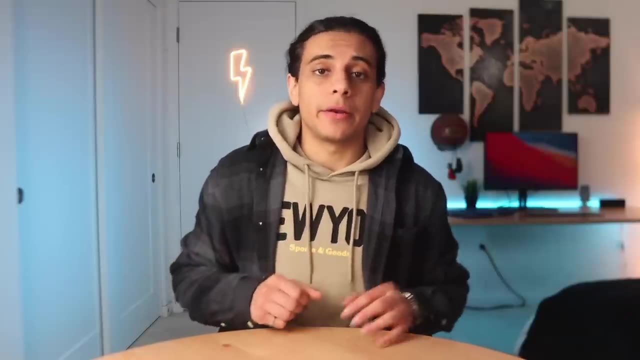 may be under a lot of direct sunlight, then a potential issue is that the adhesive may become less sticky, delaminate or change its color over time. With that in mind, you may want to implement another kind of mounting solution that isn't using adhesives. Now, after the engineering design, 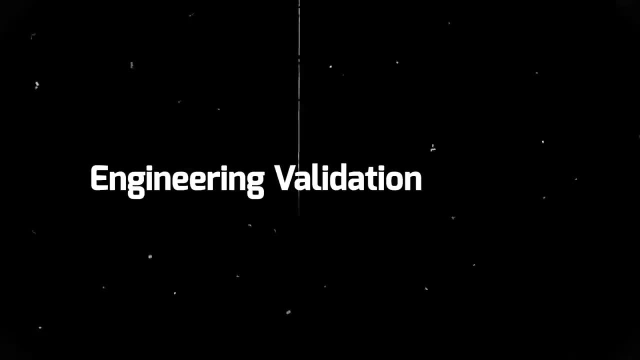 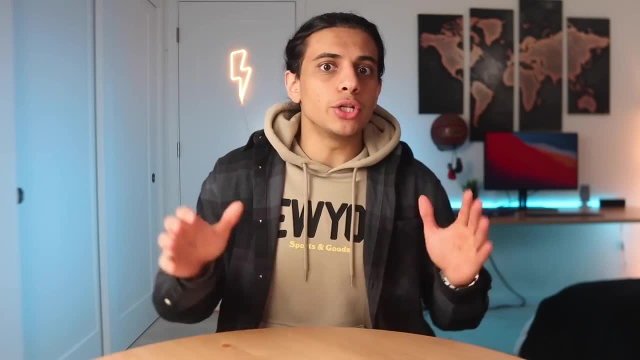 process is over and you have a working prototype, you may have to undergo the validation process. Here, you need to make sure that the design is going to do what it's supposed to do. especially if you're making hundreds of thousands of these, This process can be. 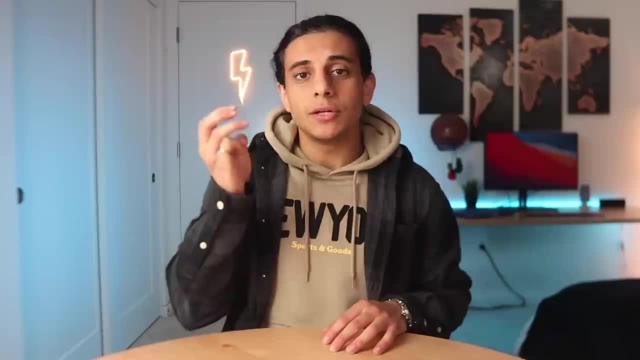 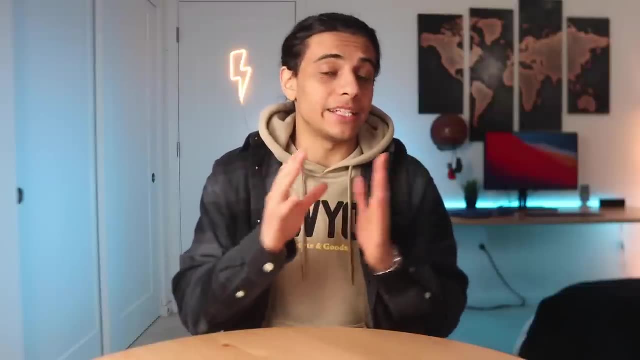 broken down into five steps: EVT, DVT, PVT, RAM and mass production. You see, engineers really love their acronyms, so what I just said may sound a little bit like gibberish, but let me explain what each step stands for. EVT stands for Engineering Validation Trial. The goal here is to 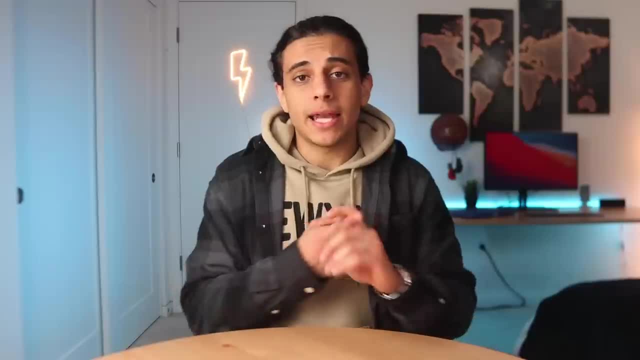 finalize the design and to comfortably build 20 to 50 units that have the desired look and actually work. But as these three steps go on and on and on, you'll need to make sure that the design is going to do what it's supposed to do. Once these units get built, about 40% of them will fail for a 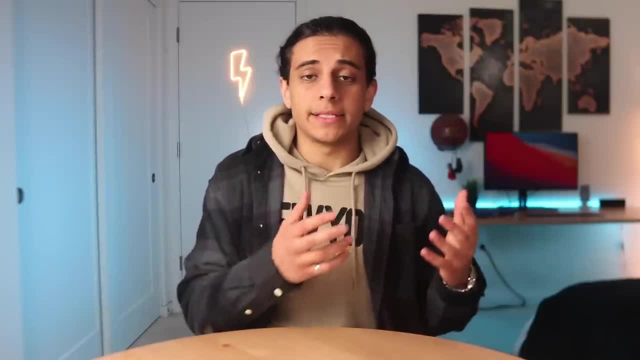 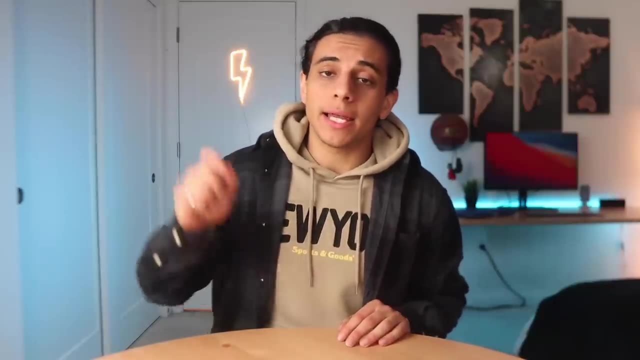 bunch of reasons. So we'll solve the issues that come up by making some slight design changes or by altering the manufacturing process that we were planning on going with in the beginning. Once the hardware is ready, it's time to move on to the next stage, which is DVT. 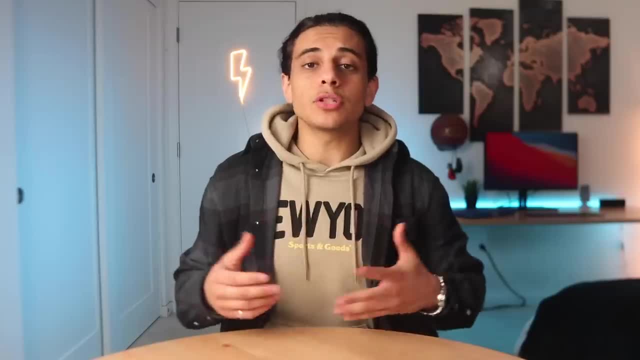 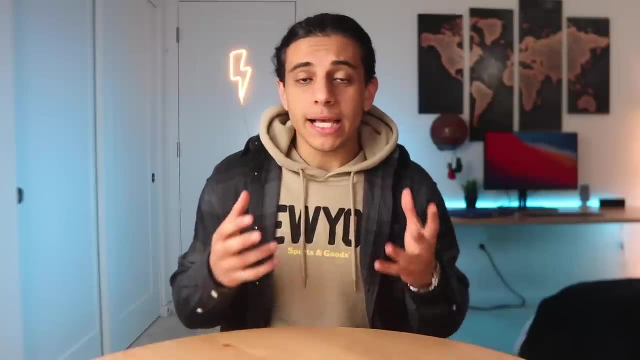 DVT stands for Design Validation Trial. In this stage, we'll focus on perfecting the tools and techniques that will actually build our part. The outcome of this stage should be anywhere between 50 to 200 units that are actually built using a proper manufacturing process. These units are: 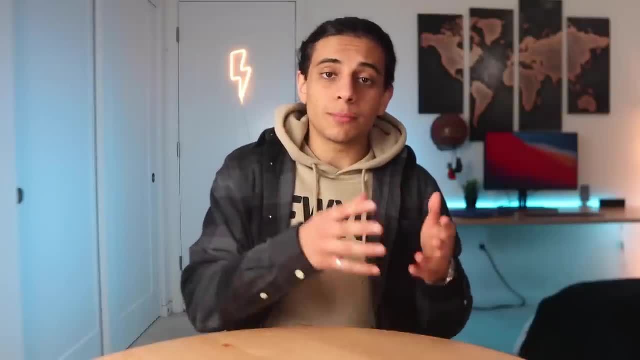 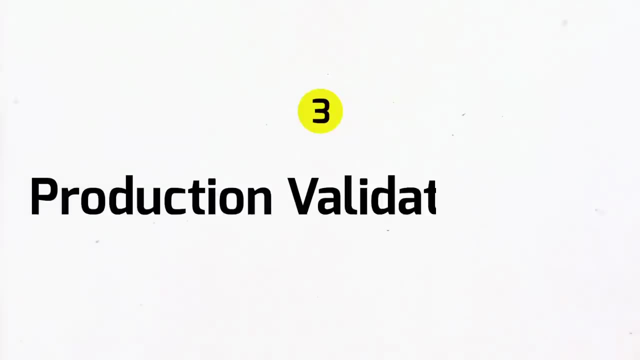 designed to be durable and reliable. Now, once the tools and processes that we're going to use to actually build our part or our product are ready, we move on to the next stage, which is PVT- PVT stands for Production Validation Trial- where every part that comes out should be passing. 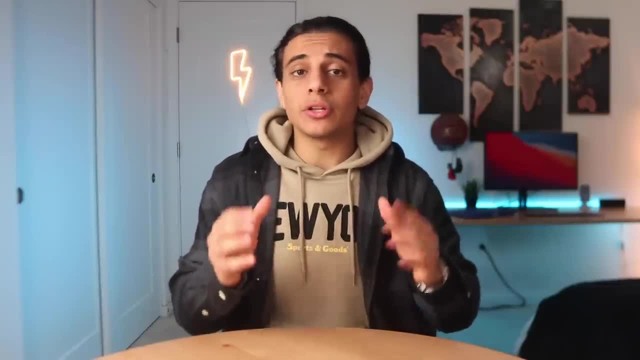 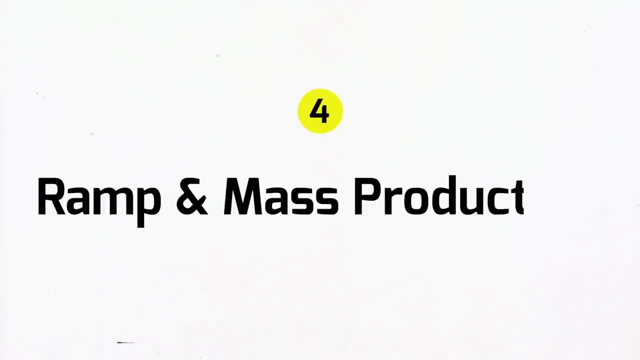 all tests and should be good to sell, But at this stage there's still some quality control procedures that the manufacturing plant will have set up to make sure that there are truly no failures. Finally, we move on to RAMP and Mass Production where, at this point, we're building: 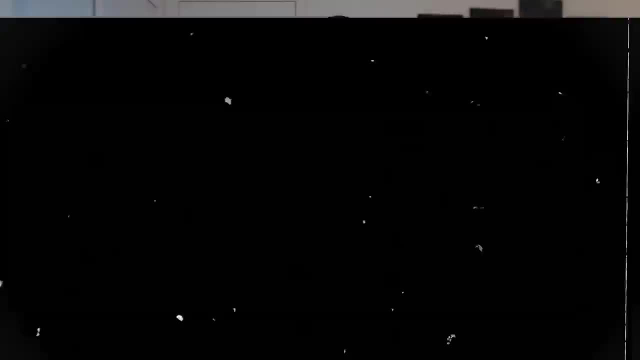 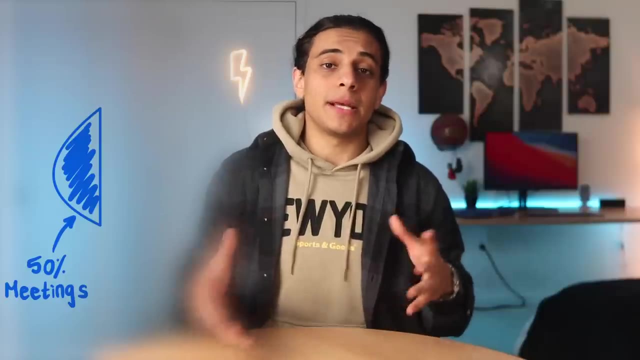 thousands of products, and the process should be streamlined by now. If I have to break down my job into how much time I spent doing all the different things I mentioned so far, I'd say about 50% of my time is spent in meetings. then about 25% of my time is spent designing where I'm 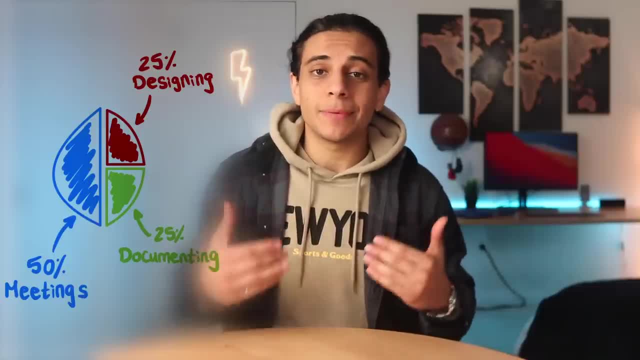 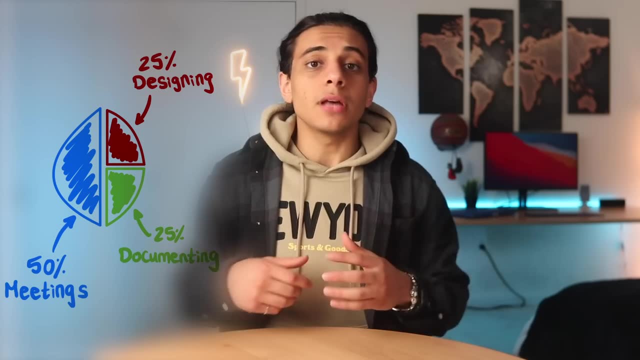 just working in SOLIDWORKS. Finally, the remaining 25% is spent documenting my work. That means I could be creating documents explaining why I made a certain design change, or maybe a document talking about how all these different parts would be assembled together. Anyways, I hope this video.